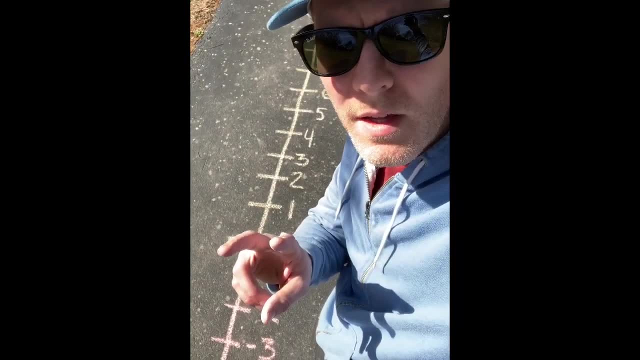 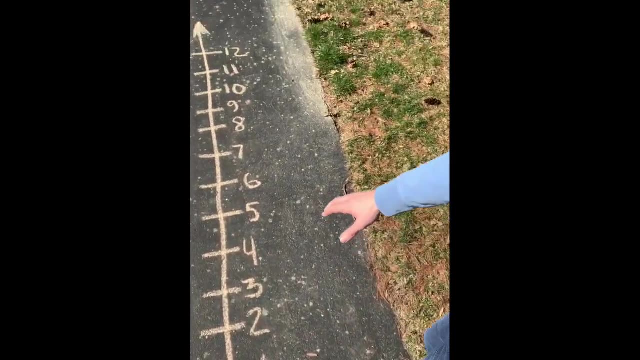 are and how they work. Okay, so really, there's two ways to think about a number line. One of them is what's called a vertical number line. This is where you have zero in the middle and as you move up, you have what's called positive numbers, And then those are the numbers you 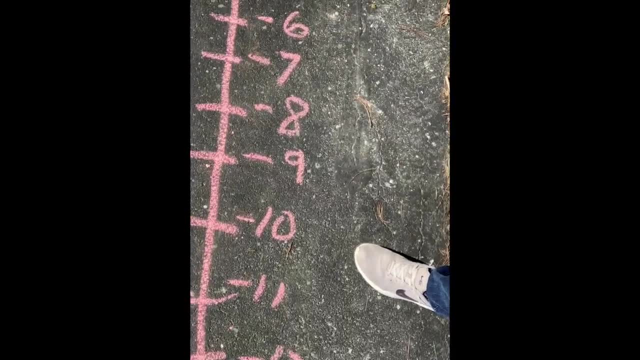 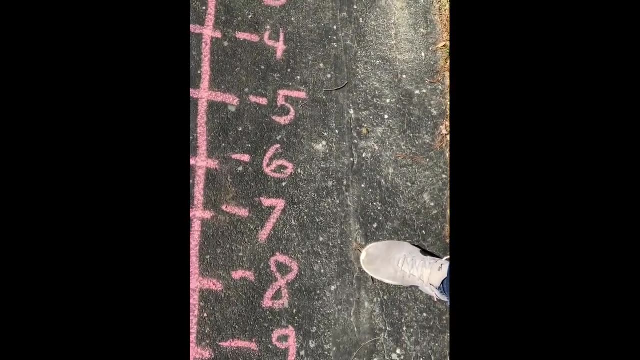 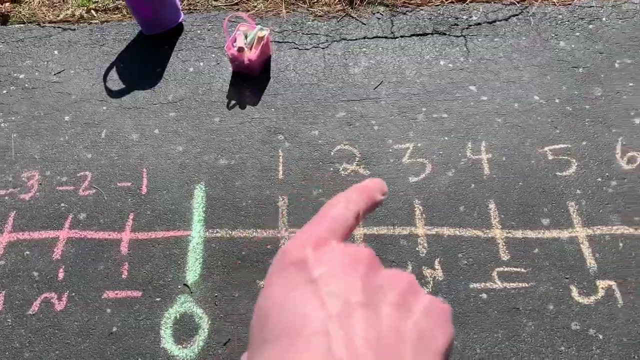 already know, And then, as you move down, you have negative numbers. This is a vertical number line with positives going up and negatives counting downwards. The other way to think of it is a horizontal number line where the number, the positive numbers, count up in this direction. 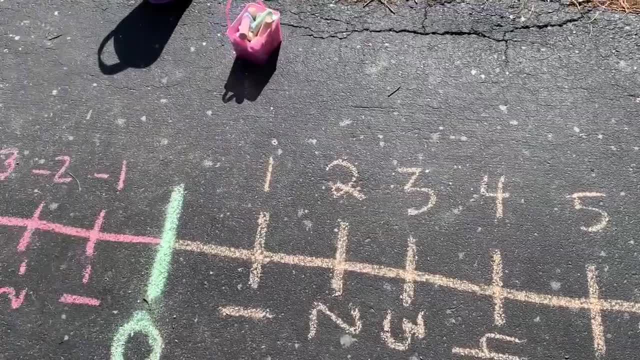 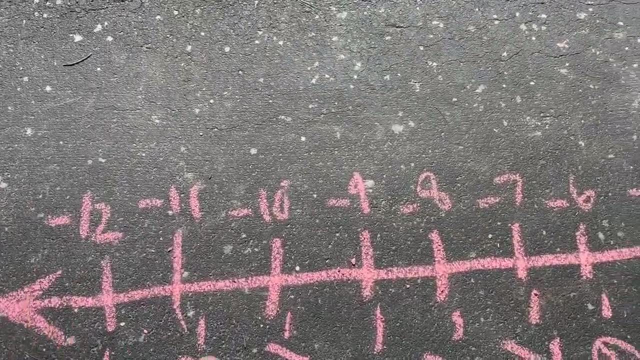 the direction we're used to, And then the negative numbers are counting in the opposite direction. negatives and positives count in opposite directions, So this would be a horizontal number line with zero in the middle, Probably one of the most important things to realize about. 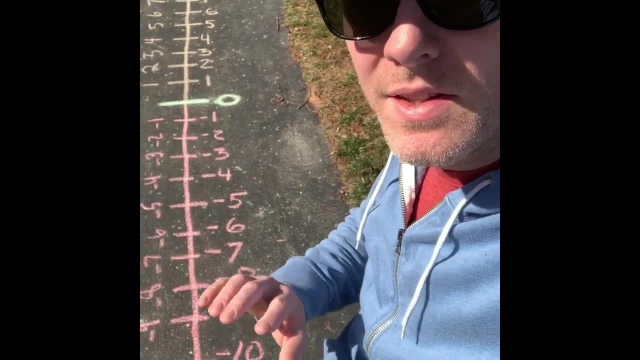 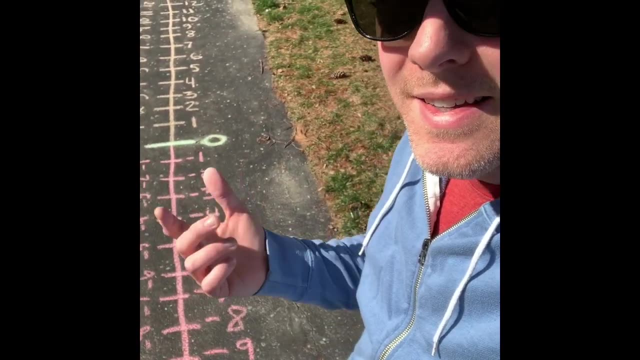 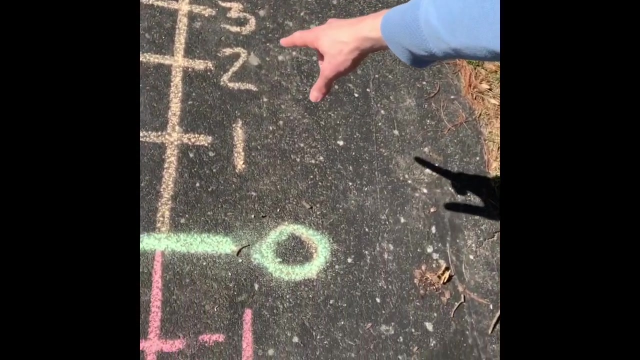 negative and positive numbers is that they're completely different. The number 2 is a completely different number from the number negative 2, and in fact they're four away from each other And if you look you can see positive two is four spaces away from negative two. 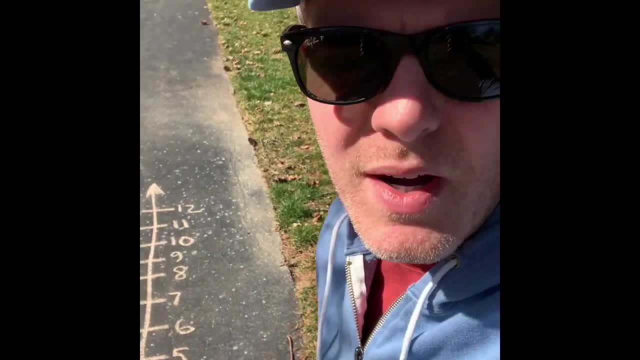 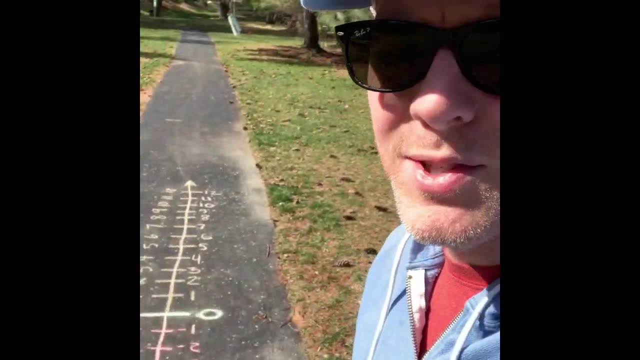 Because negative two is two under zero and positive two is two above zero, So they're actually four away. So whenever somebody says: oh, the answer was supposed to be negative two, but I put positive two, I just forgot the negative sign. 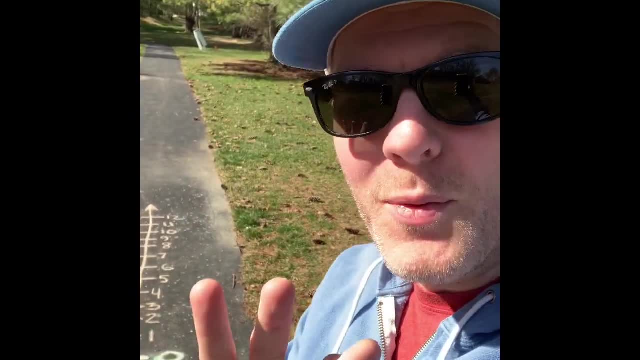 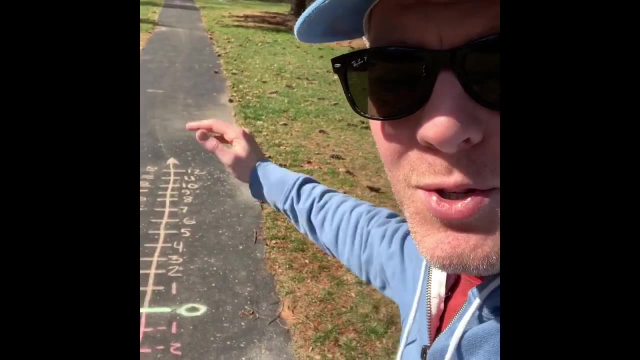 Well, you put a whole different number down because you're four away from what the answer is supposed to be. And think about 12.. If you put 12 down but it's supposed to be negative 12,, well you're 24 away from what you were supposed to get. 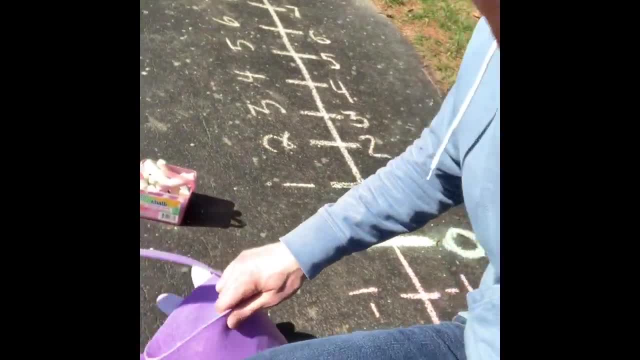 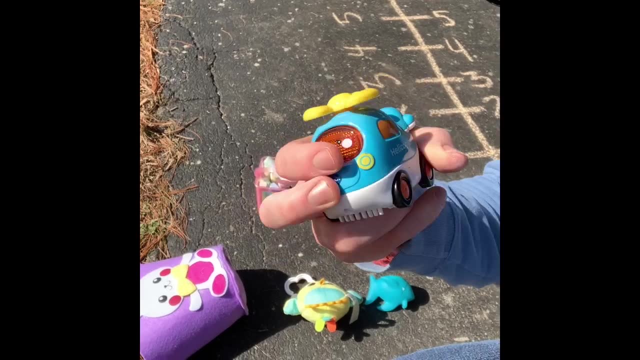 because negative 12 is way down here And I decided to steal some of my son's toys here to help illustrate some points. So we have a little helicopter here. I think it makes noise. There it goes. Oh, it makes a song. 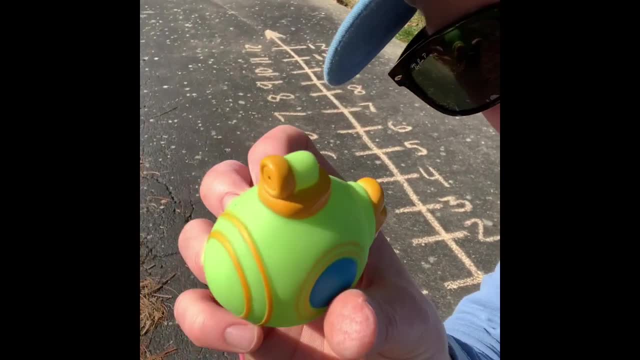 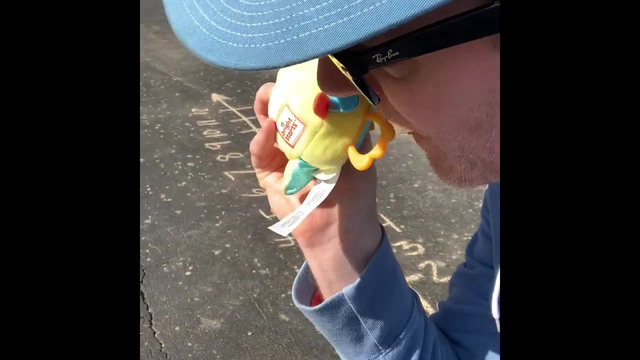 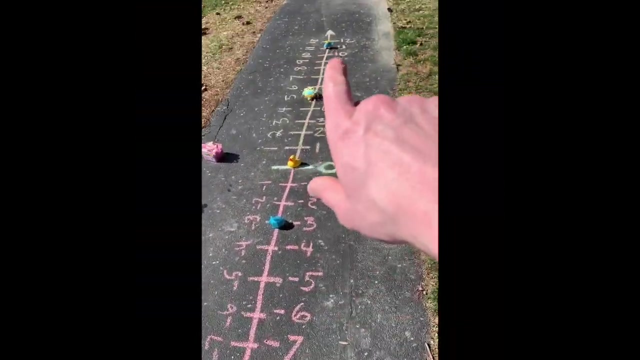 We have a shark, And then we have a submarine And a rubber ducky, And This one's nice. It's a, A bird On my number line, whether you want to see it vertically like this, or, of course, you can see it horizontally like this. 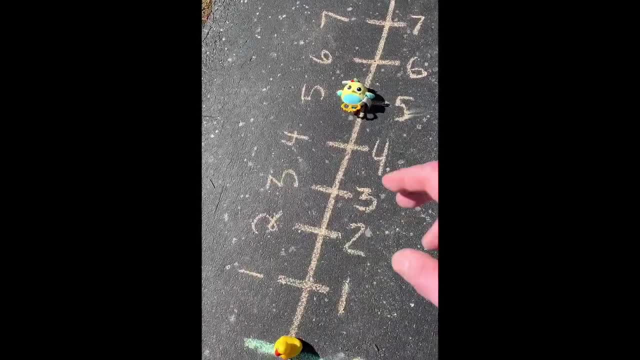 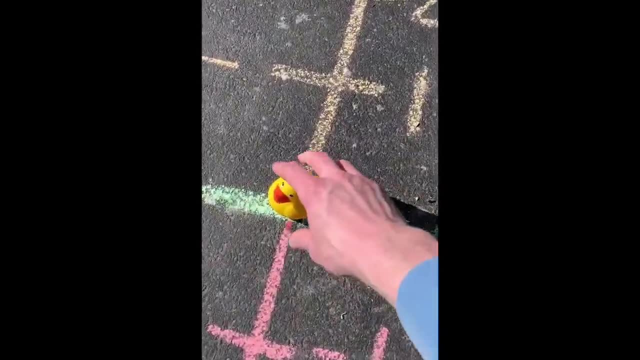 So I'm going to go with vertically. So, and the reason I'm doing that is because I have two things that are in the air, So that would represent positive numbers. I have my rubber ducky, which is here at zero, floating on the surface of the water. 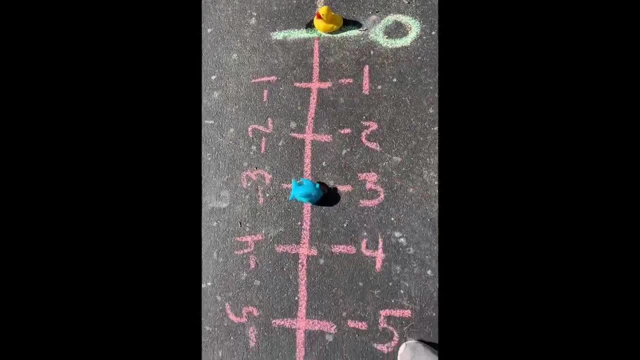 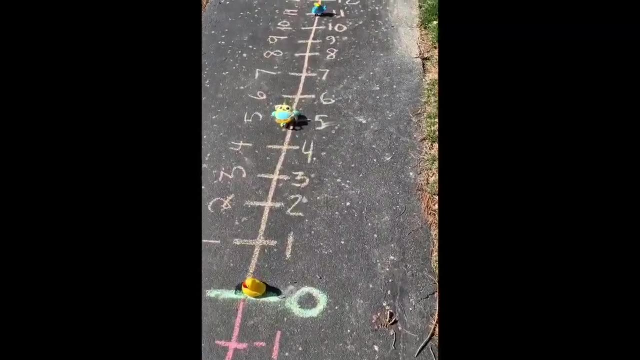 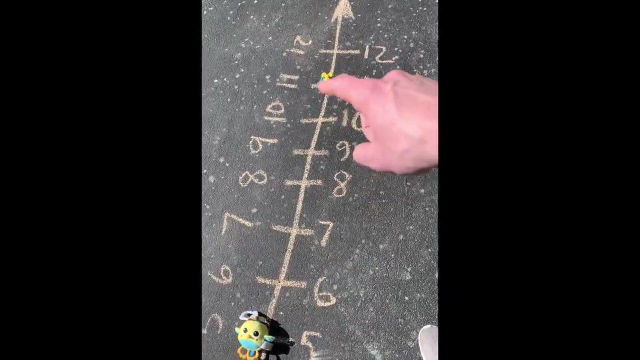 I have a shark here that's at negative three, And then down here I have my submarine floating at negative ten. So if we think about positives, you can think about how the bird and the helicopter, how far apart they are right. 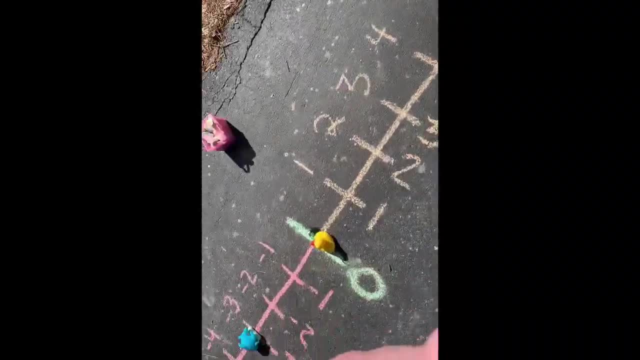 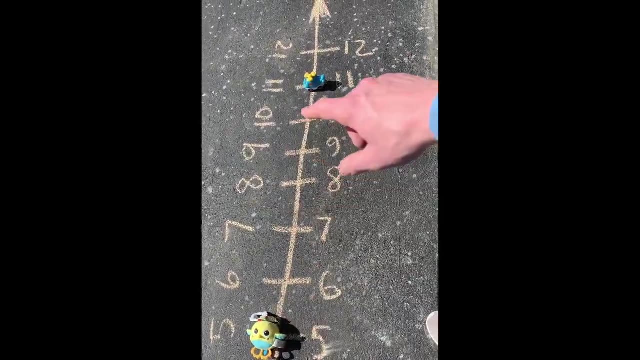 So the helicopter, which is the highest thing in my set, is at 11.. And the bird is at five. So if I wanted to look how far apart they are, you could just subtract to get six, or you could count on the number line. 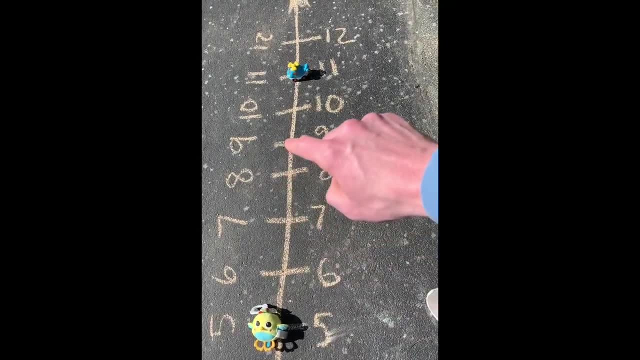 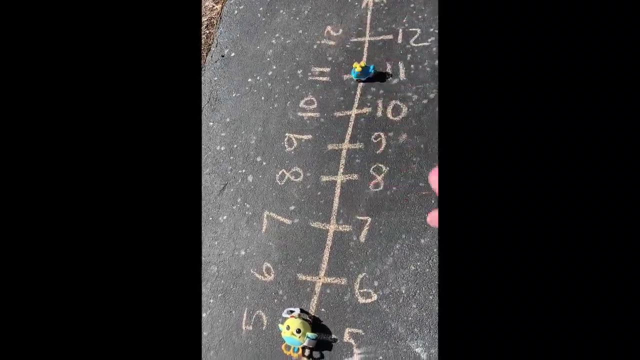 moving from the bird, one, two, three, four, five, six, So they're six apart. Of course you could just do 11 minus five to get six, and that's positive numbers. But when you get down into the negative world, 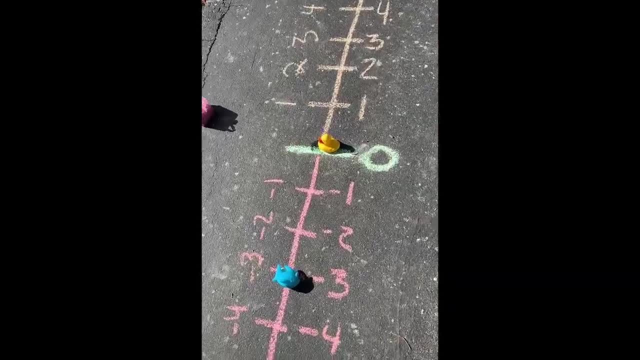 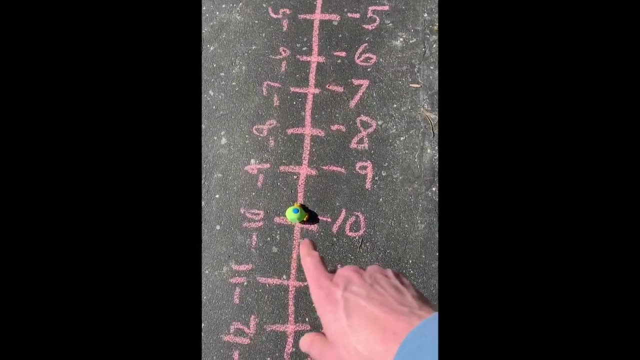 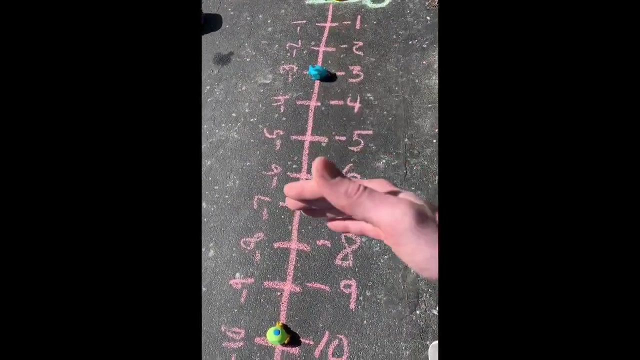 it's similar but it's a little different. So here my shark is at negative three and my submarine is at negative ten. So if I wanted to subtract, it gets a little tricky because you're dealing with negatives. But if I said, hey, how far apart are these things? 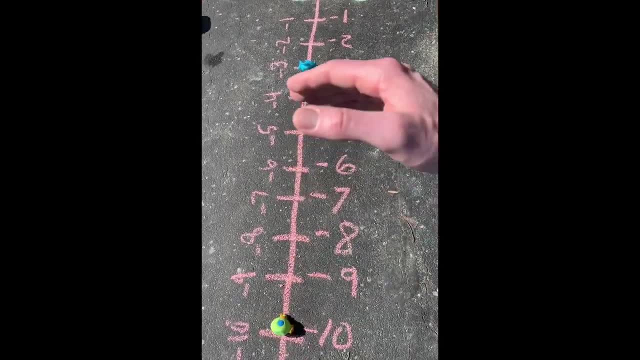 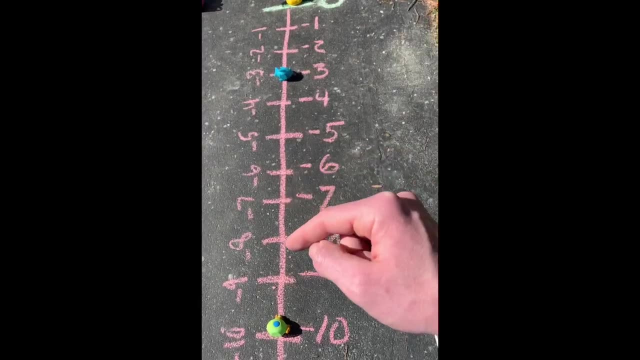 You could do the same thing on the number line. Just count from negative ten and negative three. So I'll actually count down from the shark. So I'll go one, two, three, four, five, six, seven. They're seven apart. 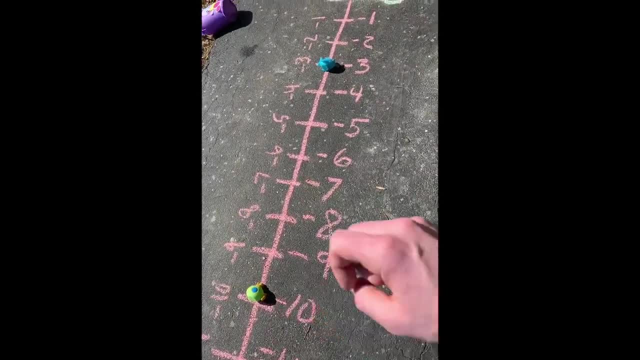 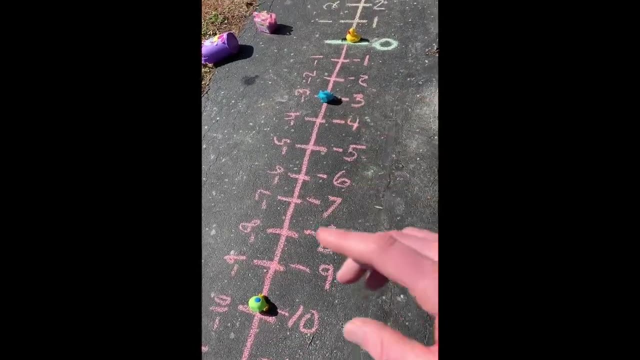 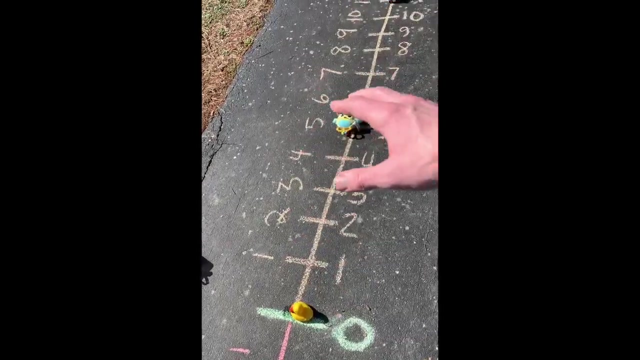 which makes sense because negative ten and negative three are seven apart, just like three and ten are seven apart. They're the same distance. But where it gets really crazy is when you start to think about how far apart things are that are negative and positive. 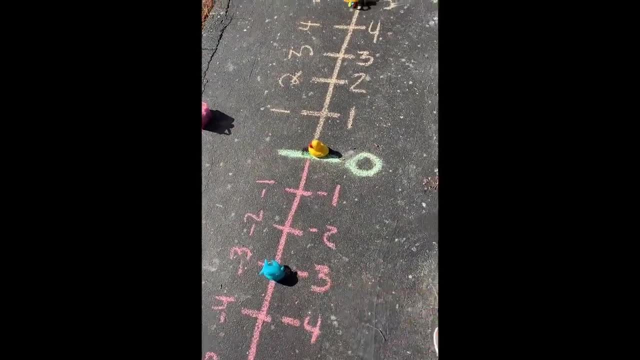 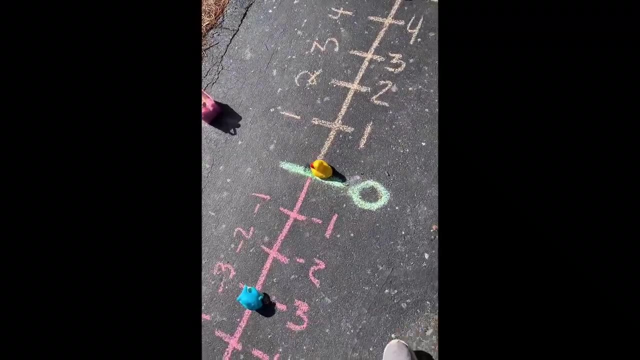 So, for example, my shark here is at negative three and my bird is at negative five. So if the shark wanted to jump up to eat the bird, then how many feet- let's say these are feet- would it have to go? 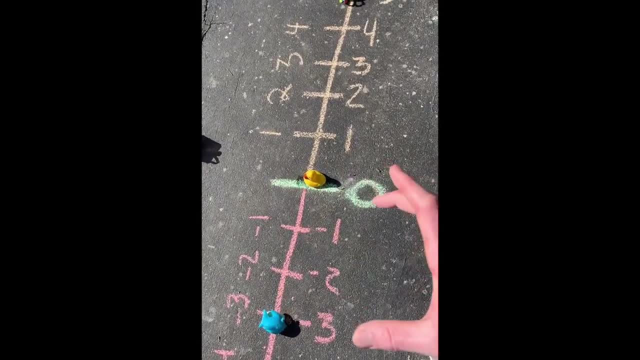 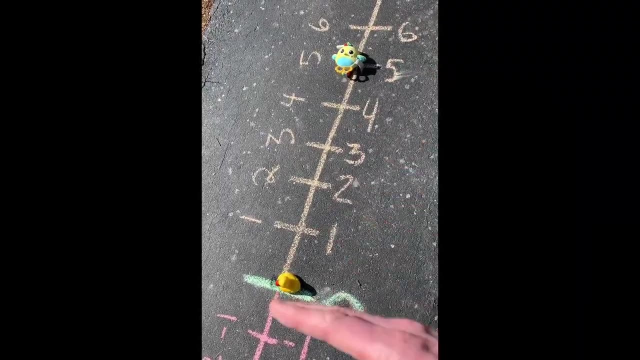 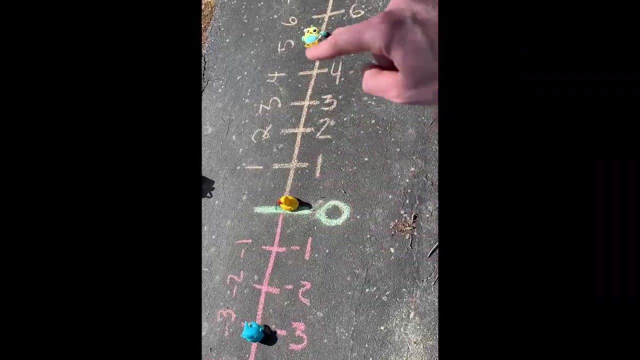 And we have one, two, three to get to zero, because that's negative three to zero. And then you have another one, two, three, four, five, so that's five from the surface to the bird. So altogether that would represent eight. three to the surface, and then another five. 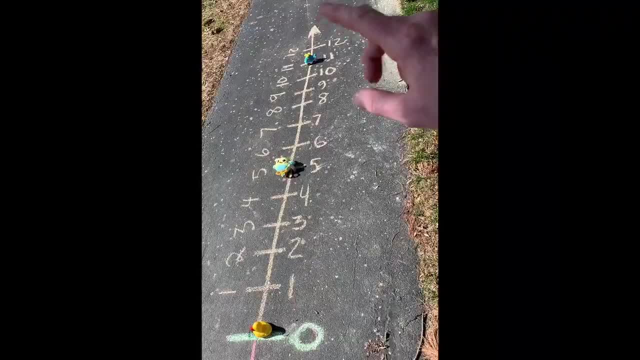 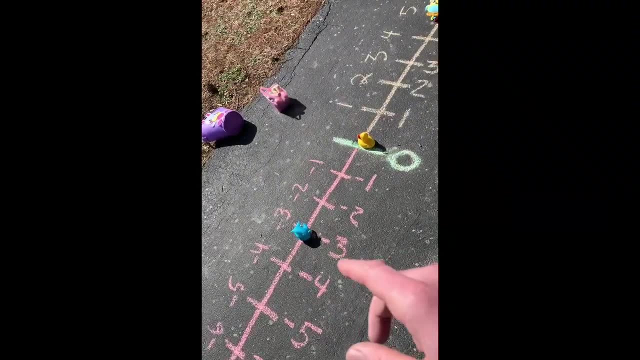 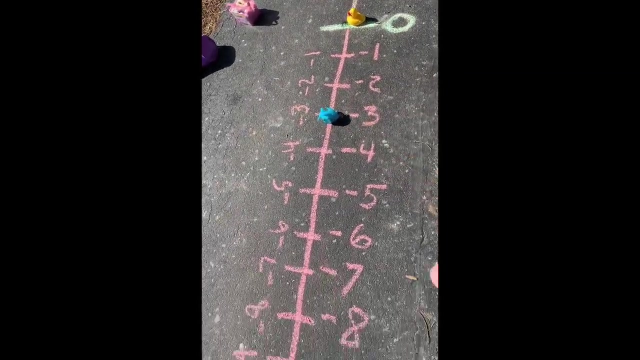 They're eight apart. And same thing with if I take my helicopter and I take my submarine submarines, the lowest thing here- at negative ten, lower than negative three, which is that's another thing. Negative three is a higher number, The negative ten, which is weird to think about, because in the positives 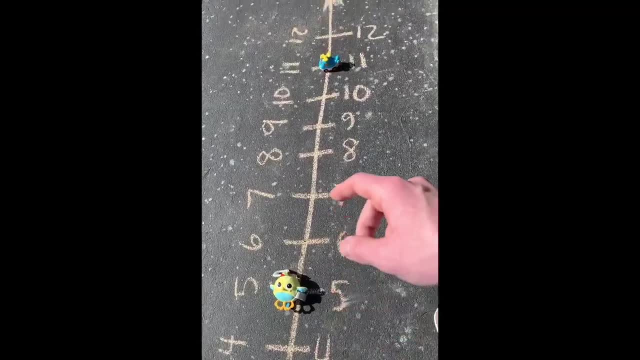 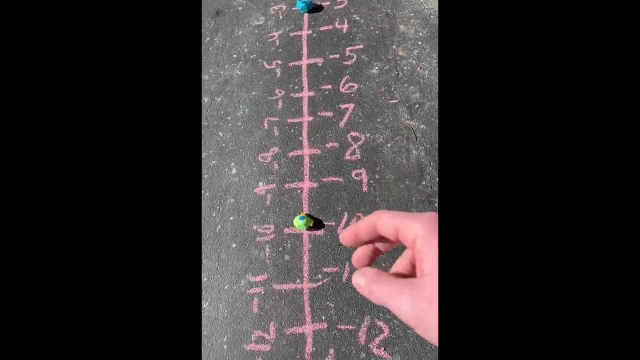 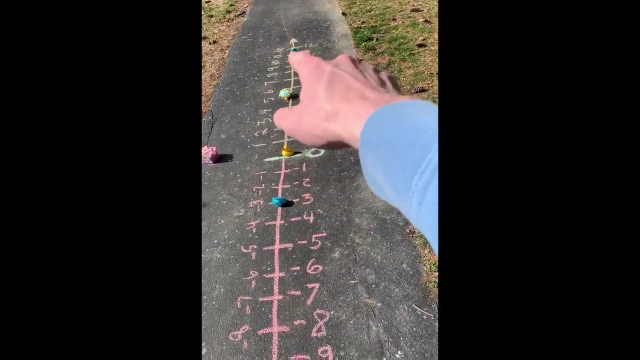 this kind of different. like the number three is lower than ten, Ten is a higher number, but in negatives everything's opposite. So negative three is actually higher up on the number line than negative ten. So if I wanted to figure out how far apart the submarine is from my helicopter over. 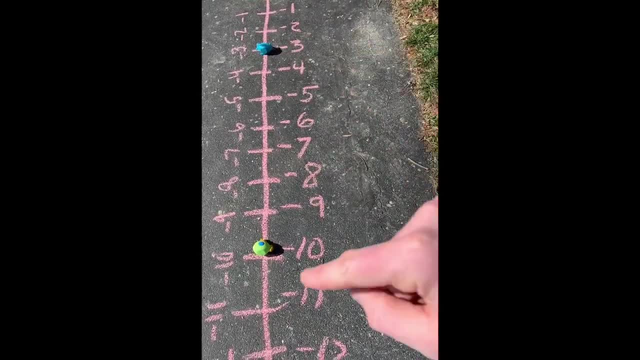 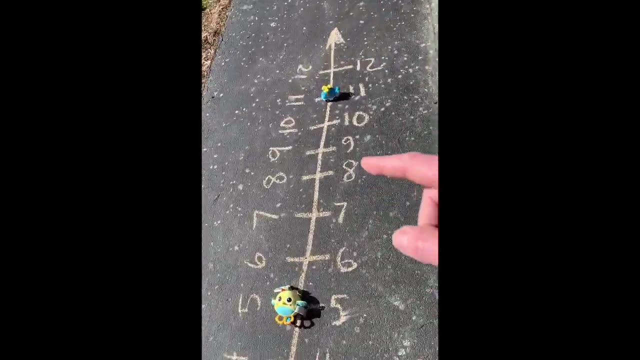 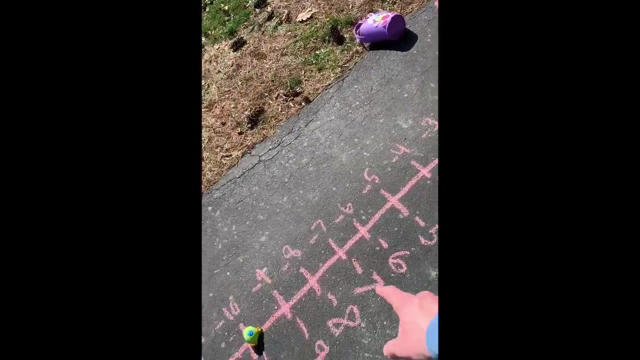 there. well, I would count up to the surface first. So ten to the surface is zero negative. ten to zero Negative three is ten, and then it would be another eleven to get to my helicopter. So all together, eleven and ten. those things are actually twenty-one apart. 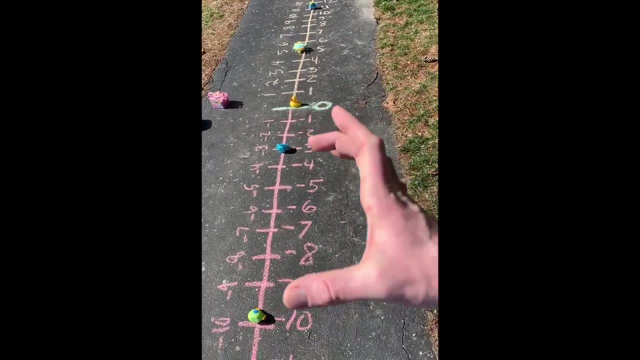 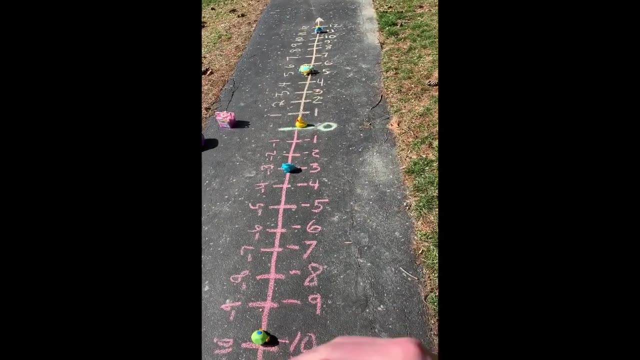 So this sort of illustrates the point about how sometimes you're thinking like three and ten, negative three, negative ten, they're actually seven apart. but negative ten and positive eleven, those are actually seven. Negative three, negative ten, those are actually seven. 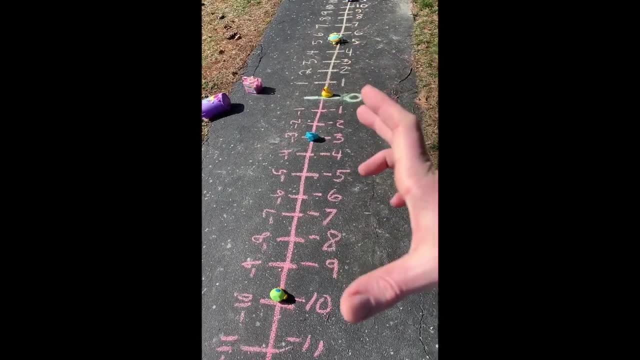 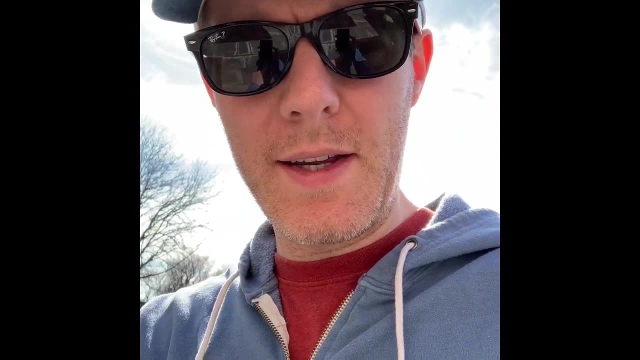 Negative three, negative ten. those are actually twenty-one apart when you combine their distances to zero. Well, that's all I got for you today for positive and negative numbers on the number line. I hope this helps. Good luck out there and I'll see you in class. 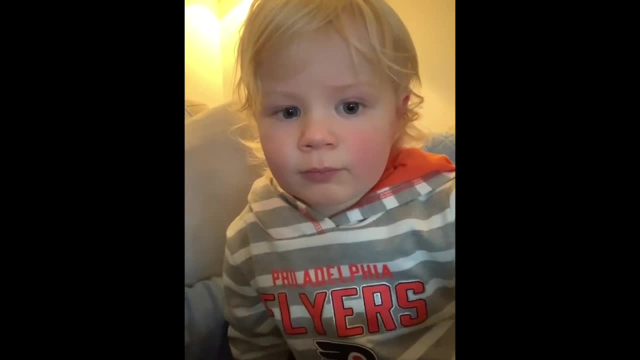 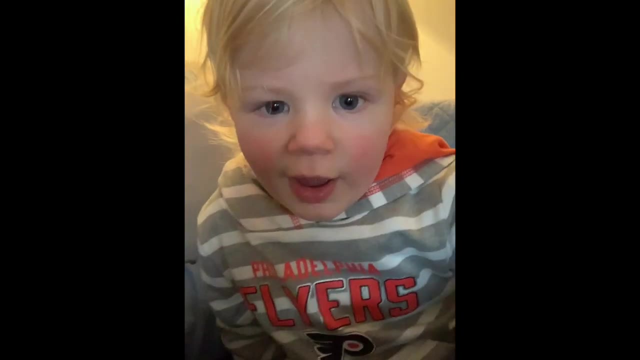 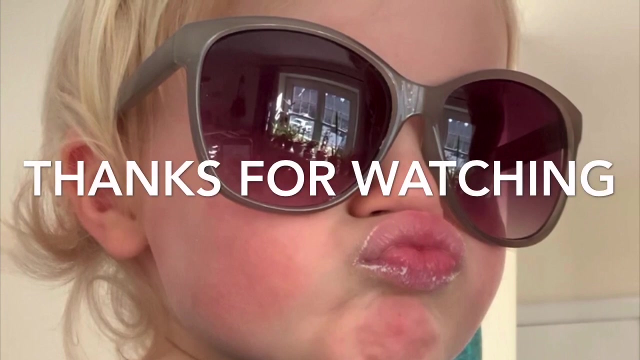 Dylan, I used some of your toys today when I was outside. Is that OK, Outside again. You want to go outside again? Yes, I'll be right back.